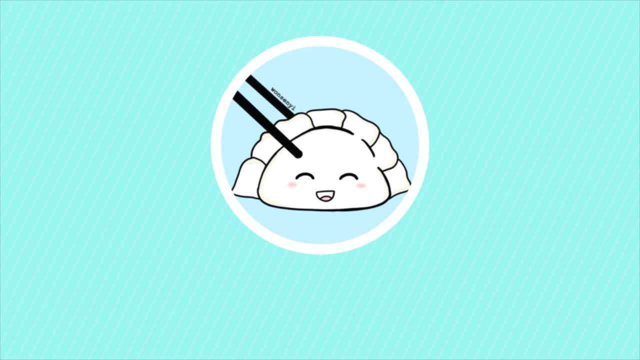 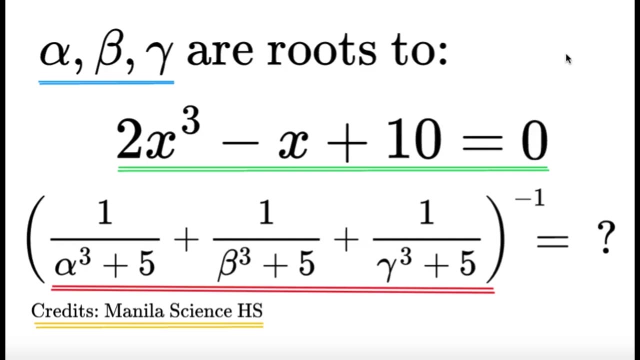 Hello, hello, It's Template here. Here's an item on algebra. Alpha, beta and gamma are roots to the following cubic equation: 2x cubed minus x plus 10 is equal to 0.. Find the reciprocal of 1 over alpha cubed plus 5 plus 1 over beta cubed plus 5 plus 1 over. 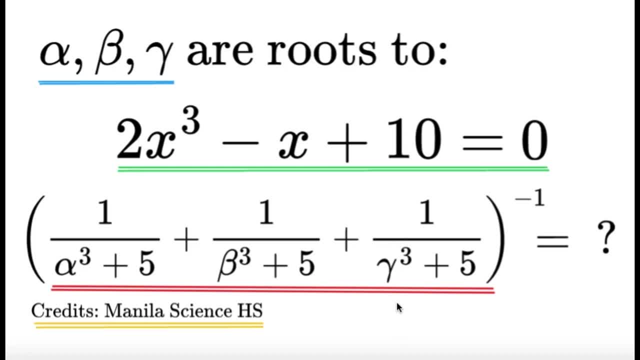 gamma cubed plus 5.. As usual, pause this video if you'd like to give this item a try, but if you're done, let us dive into the solution. Alright, so this question is one of those classic questions where we're given with an equation and we're 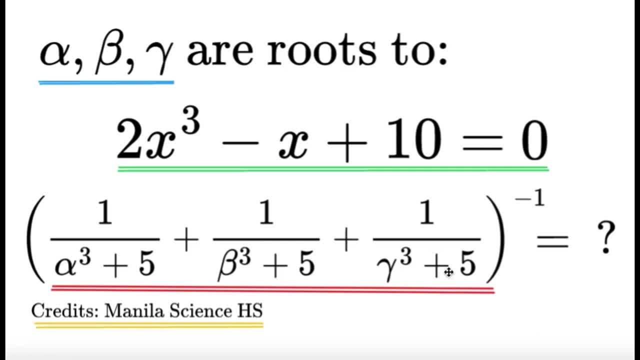 going to solve for a specific expression. In this case, we have this one highlighted, highlighted in red, and it is expected that we are not going to solve for the roots, because I am pretty sure the roots to these, to this equation, are not easy to get. so we are going to use probably some algebraic manipulation and 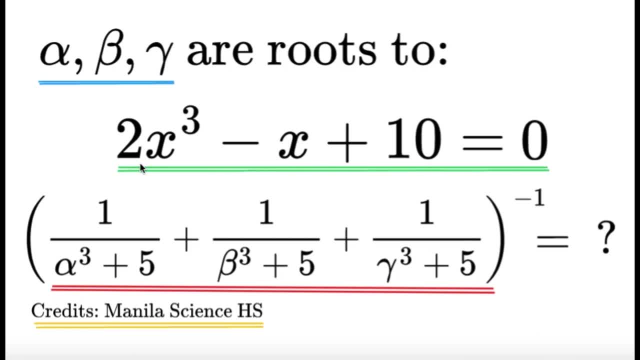 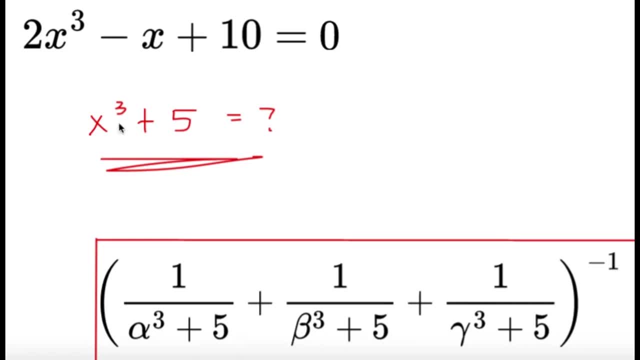 ultimately the Vieta's relations to kind of help us get the specific values that we need. Well, but the problem is, from the given equation and the expression that we want, I mean, it's impossible for us to get what x cubed plus 5 is so there. 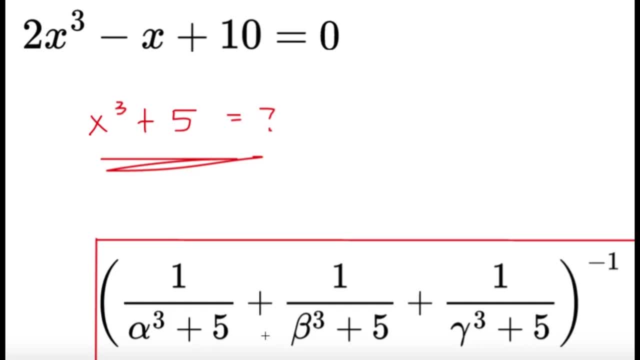 isn't really a nice way to tell us what the alpha cubed plus 5, beta cubed plus 5, gamma cubed Plus 5 is, unless we write it into something else, because, well, there isn't really a direct formula to tell us what this part is. So we know what we can get from Vieta's: the sum of 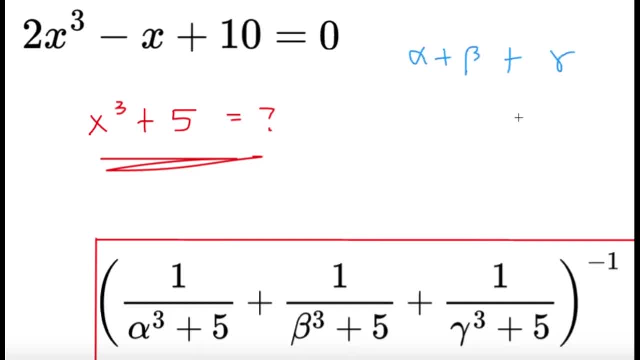 the roots we can get. we know what this is and we know what this is: the sum of the product taken as the sum of the roots, taken two at a time, and we would know what this thing is. So these are the only three values that we can. 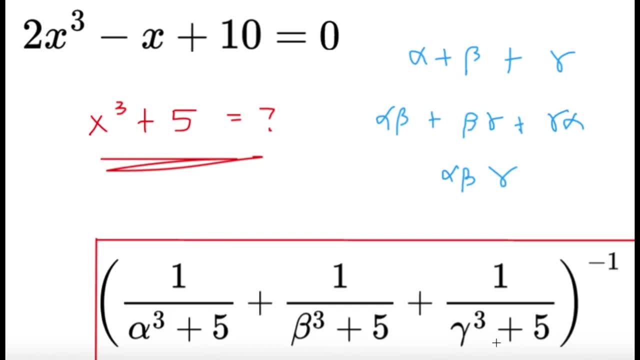 get from Vieta's formula, so we have to probably write it into real kim嫨, this in terms of something else. So we're going to use some algebra first to kind of help us get what x cubed plus 5 might be, because that's the format of the denominators. So 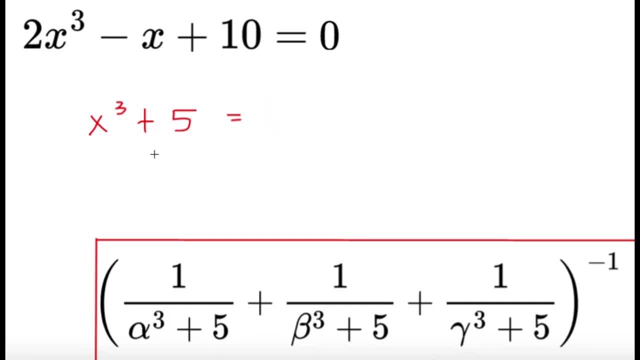 all right, let's try to manipulate this given to get x cubed plus 5.. Now what's pretty nice here is that, well, 2x cubed and 10, I can factor the 2 out and I'll get x cubed plus 5 that way. So 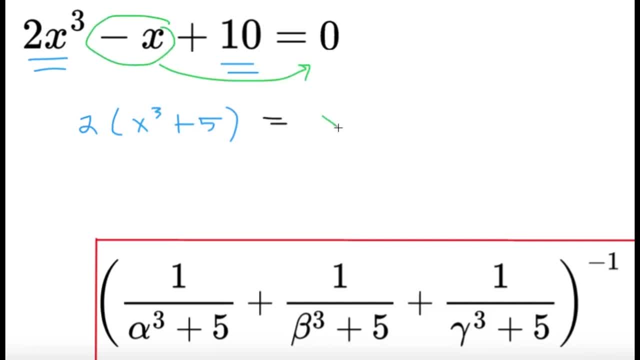 apparently if I move the x to the other side. so I'll have the following relationship: 2 times x cubed plus 5 will be equal to x, and then, dividing both sides by 2, x cubed plus 5 is equal to x. 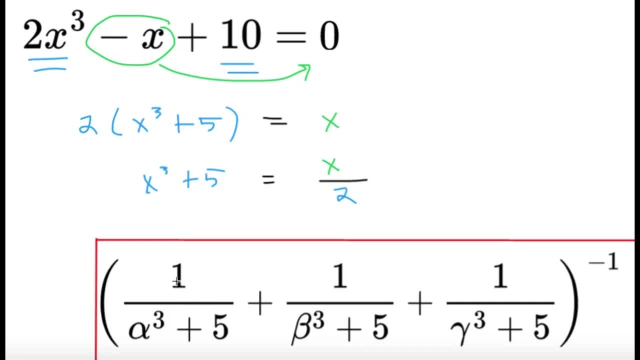 divided by 2.. So I think 1 over alpha cubed plus 5,, 1 over beta cubed plus 5, 1 over gamma cubed plus 5, well, we have to take the reciprocal of this, So I'll get that 1 over x cubed plus 5,. 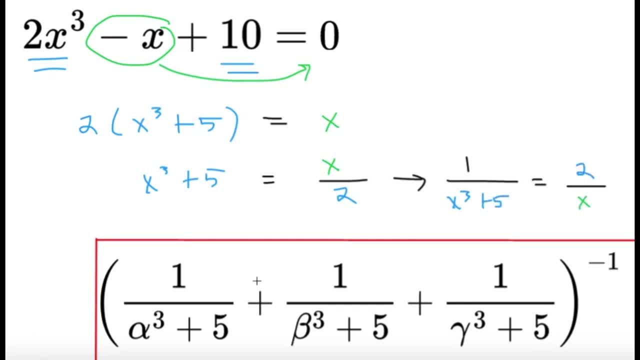 that would be the same as 2 over x. So I know that 1 over alpha cubed plus 5 is going to be 2 over alpha. 1 over beta cubed plus 5 is going to be 2 over beta. 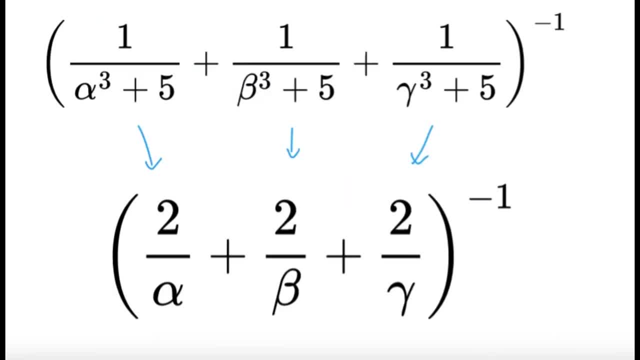 and same thing for the gamma. So this expression that we want, we can rewrite it as follows: So, as you can see, here, essentially we're just asked to get the reciprocal of 2 over alpha, plus 2 over beta, plus 2 over gamma. Now, this is a very familiar scenario. it's just the sum of the reciprocals. 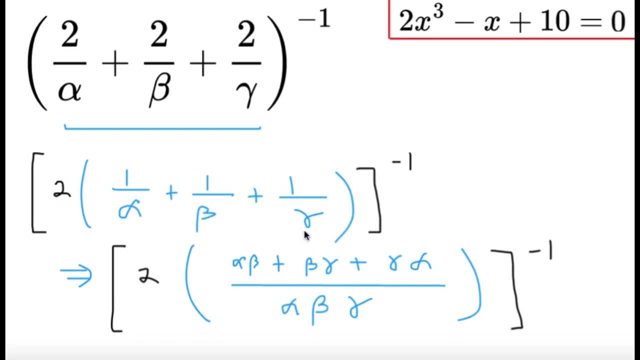 I mean, there is a factor of 2, but we can easily take care of that. But we know that the sum of the reciprocals of the roots can be expressed as this: So essentially we're just writing these three fractions, because 1 over alpha is just the same as saying beta gamma divided by alpha beta gamma. 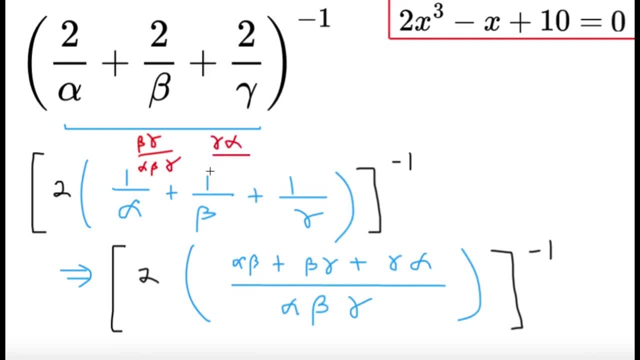 and then 1 over beta is the same as gamma, alpha divided by alpha beta gamma. and then 1 over gamma is just alpha beta divided by alpha beta gamma. So just writing it in terms of one fraction we're going to get this All right. so from the Vietas relations we get that alpha beta plus. 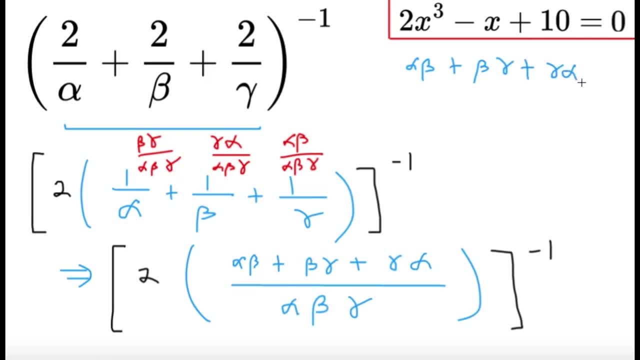 beta gamma plus gamma, That's going to be the sum of the roots. taken two at a time, That's going to be equal to negative 1 over 2.. And then for the product of the roots, alpha beta gamma, that's going to be negative 10. 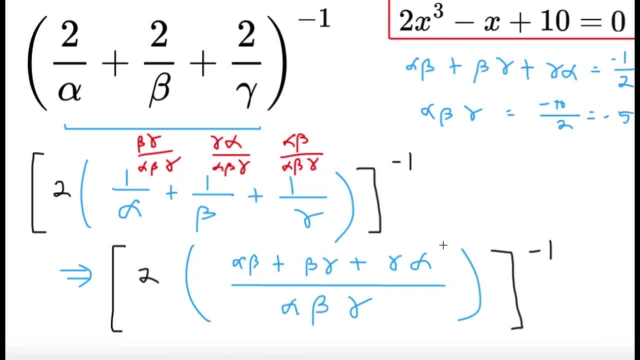 over 2, which is going to be negative 5.. All right, so the numerator here is going to be negative 1, half The denominator here. it's going to give us negative 5.. It's just a matter of substitution, So substituting the values that we have from Vietas relations. 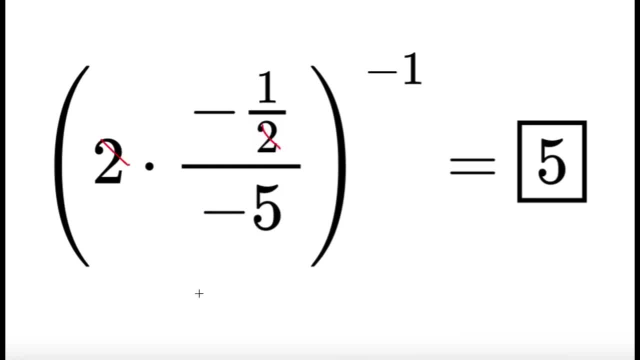 2 times the negative 1 half. here the 2 cancels nicely. So essentially it's just going to be 1 fifth, inside the parentheses. But we're taking the reciprocal of 1 fifth and that's the reason why we're going to get the final answer of 5.. And this is the answer. Hopefully you guys learned. 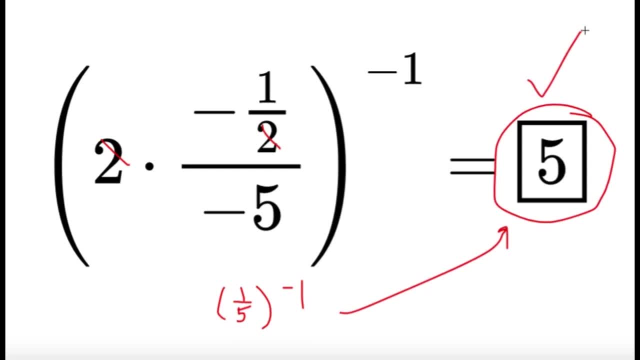 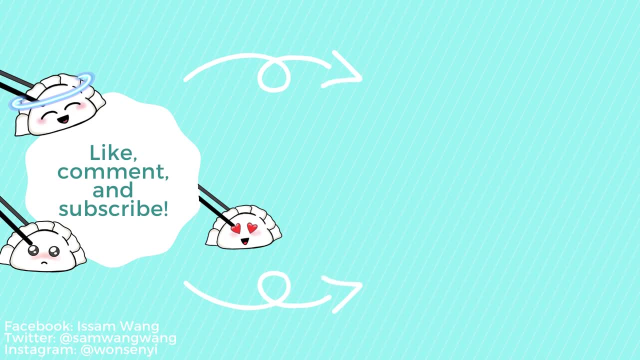 something new from this video and I'll see you in the next one. Bye-bye, Bye-bye. 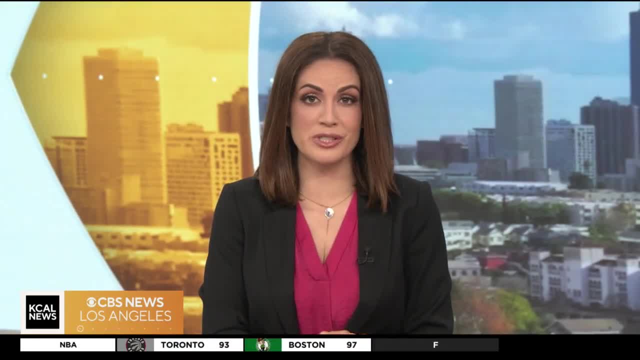 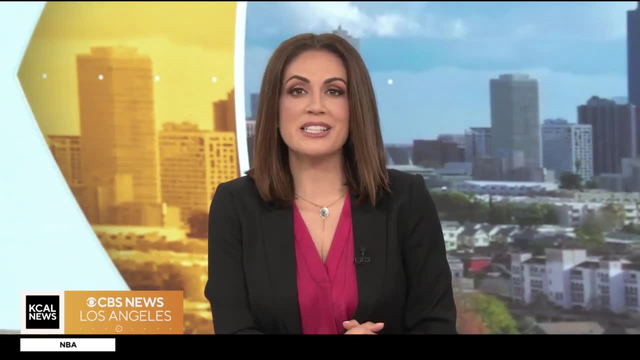 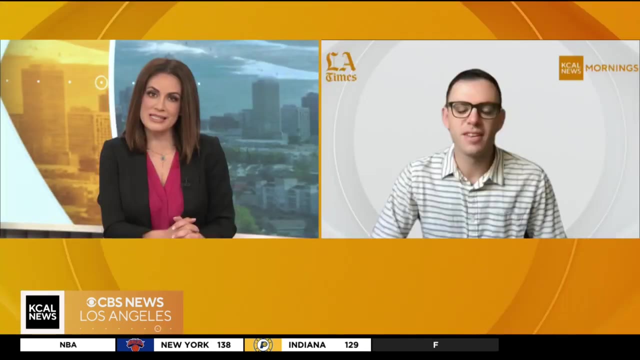 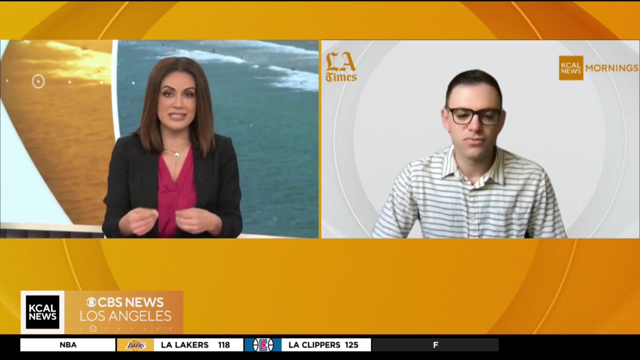 Welcome back. While California's overall population continues to shrink, new census data shows population swings have affected both large and small counties across the state. In this morning's The Brief, LA Times data reporter Terry Castleman is joining us now with a closer look. So, Terry, good morning to you. Thanks for being back with us, And you've been looking into the census data for a while now. Last time we had you on, you showed us how many people are moving out of the state, And we did talk a little bit about the shift happening within the state as well. But now you've been digging into those numbers. What have you found? 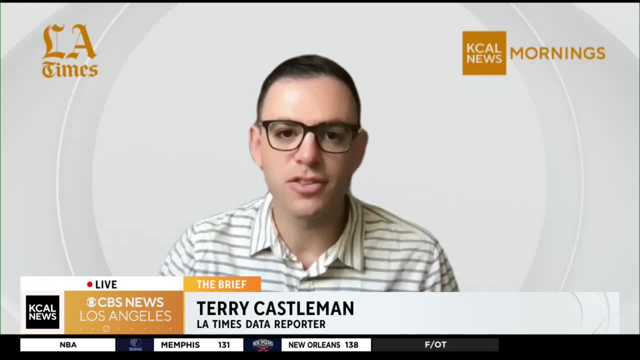 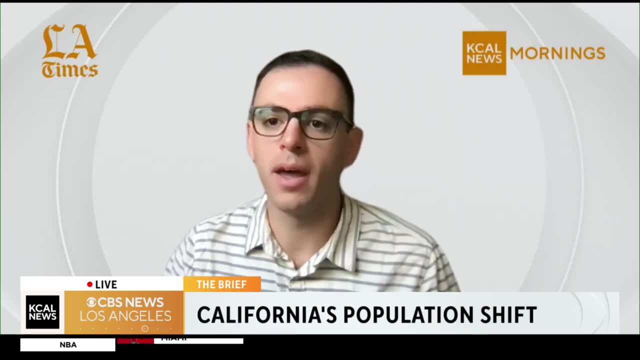 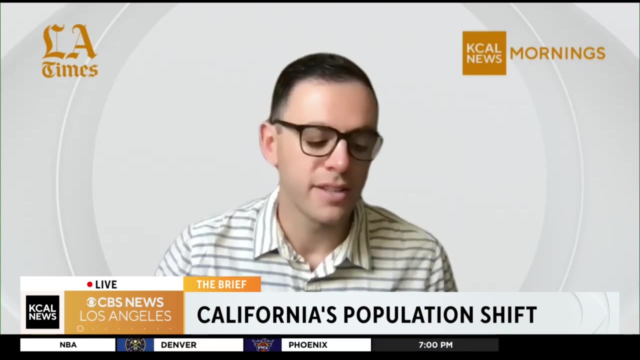 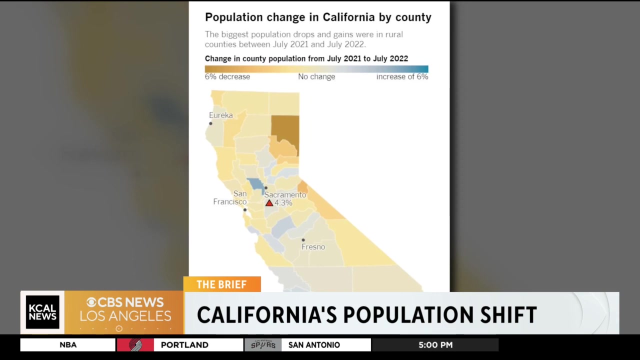 Yeah, so we've found some interesting trends about rural and urban areas within California. As you mentioned, California is losing population generally, but I was curious to dig into where exactly this is taking place And what I found is that in the most recent year, it's actually rural areas which are losing more of their population on a percentage basis than urban areas, which is in stark contrast to the year prior, when urban areas lost quite a few people. 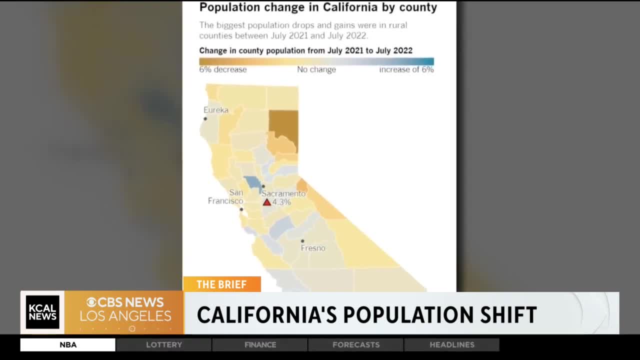 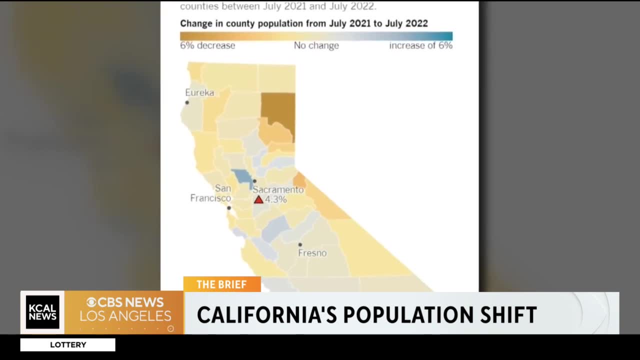 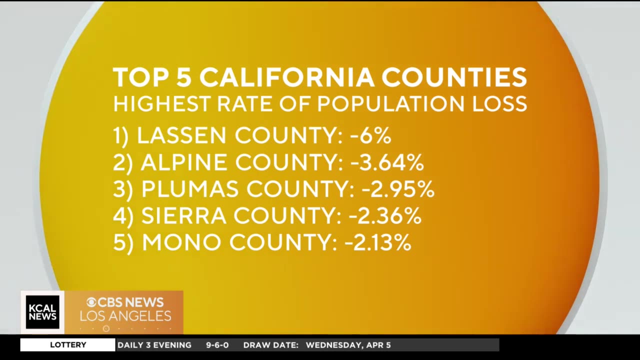 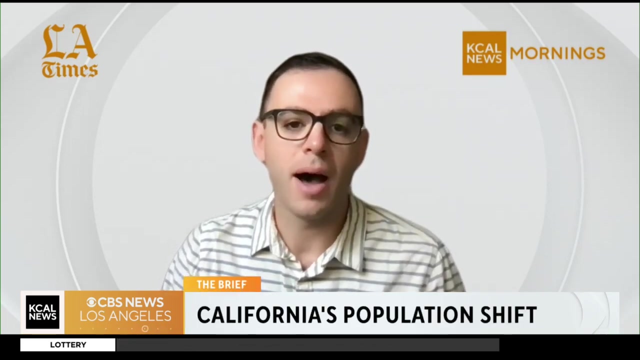 Like we talked about San Francisco, but also Santa Cruz and Santa Barbara counties, had seen tremendous drops in population. This time around we're looking at more rural areas: Lassen County, Alpine County, Plumas County, Sierra and Mono counties. These are not places you would typically think of as losing large chunks of population, but they are losing relative to how many people they have quite a number of people. In Lassen County I spoke to officials who went into the closure of a prison.